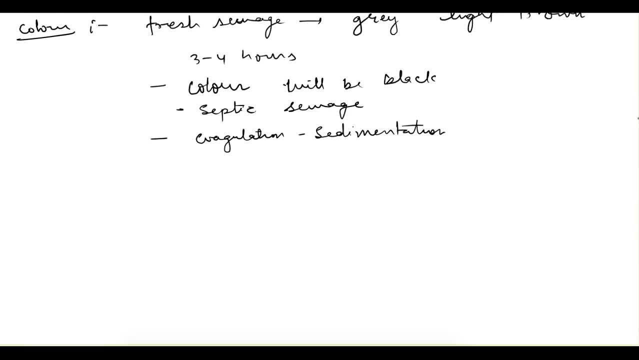 After color, the next physical characteristics we have is odor. So for the fresh sewage this odor is musty, but as the time passes, again the gases are there which will be released due to the bacterial action and the organic matter will be broken down, I mean, the decomposition of the organic matter will be taking place. So because of that, after some time this odor due to H2S, that is, hydrogen sulfide and other sulfur compounds, is released. So you can remember, initially the odor is musty and then, after the decomposition starts, that is, after 3-4 hours, this odor will be coming very strong odor will be coming from the sewage due to the hydrogen sulfide and other sulfur compounds. 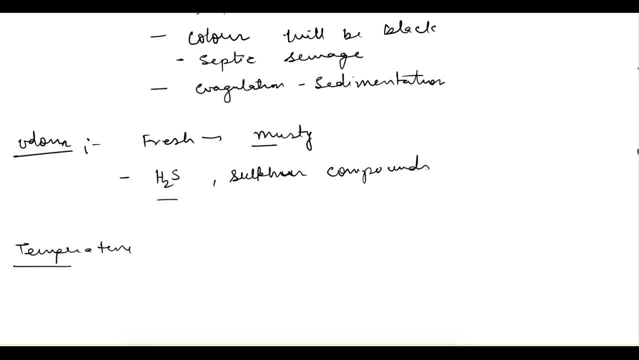 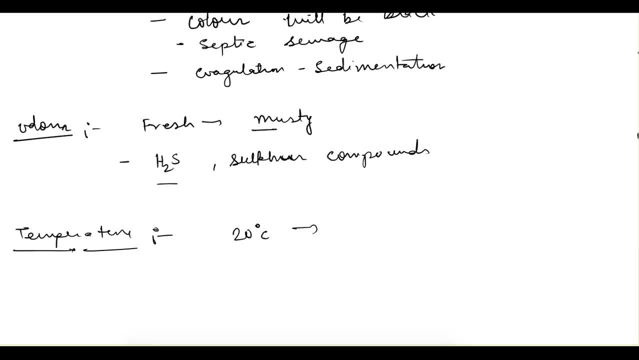 Next is temperature. For the temperature of waste water In India, this temperature is around 20 degree Celsius and which is very suitable- or we can say ideal- for bacterial activities. That is, bacteria can break down the organic compounds or organic matter, So it is ideal from that point of view. 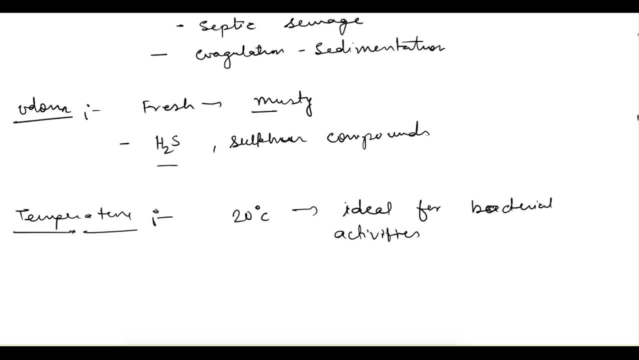 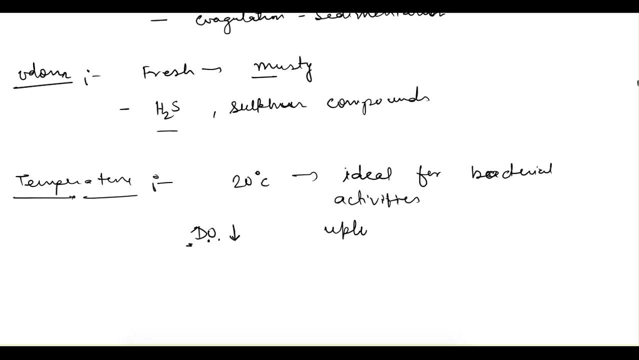 But in general, if the temperature increases. so due to that, first of all this, the dissolved oxygen that is there in the waste water, it will be decreasing, because as the temperature increases, the DO content in the water decreases. So apart from that, and this for this bacterial action, up to 60 degree Celsius. 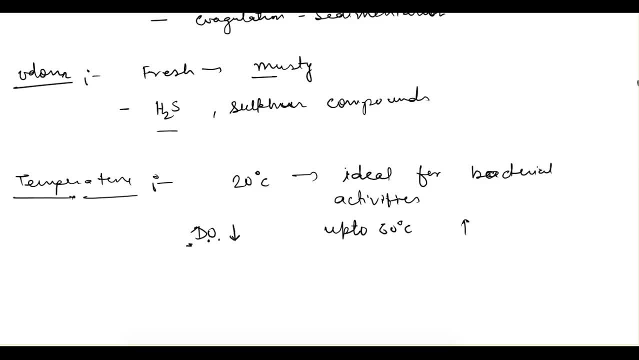 This bacterial activity increases and if the temperature is increased further then this bacterial activities will be coming down. That is for your temperature, and then we have turbidity. So obviously the waste water is highly turbid because it has different kind of impurities and suspended matter. 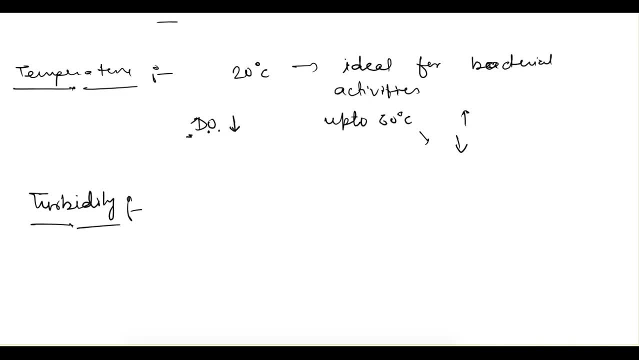 So for the measurement similar to the drinking water, it can be measured using Jackson scale, Using Jackson's turbidity meter or turbidity rod. You can remember the turbidity is very high for the waste water. These are the physical characteristics. Next we have chemical characteristics. 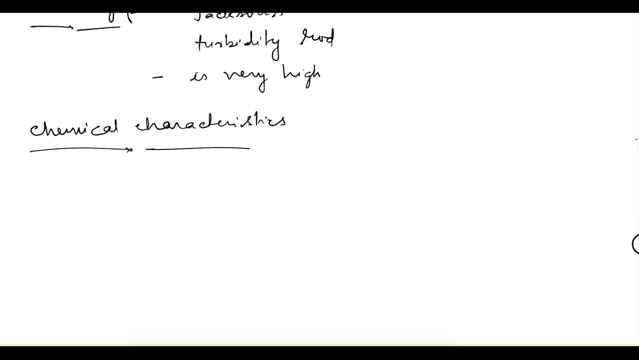 So first let's see the solids, That is, total solids, And then we have suspended solids And we can further say the settleable solids in that. So let's see all these one by one, These total solids. We can divide them into further two parts. 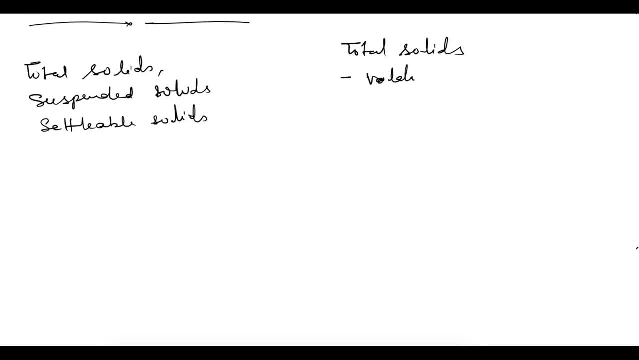 That is, your volatile solids And the fixed solids or non-volatile solids. So fixed solids are made up of inorganic matter That will consist of sand particles or gravel, Or some small glass particle may come, etc. All these inorganic matter will come in fixed solid. 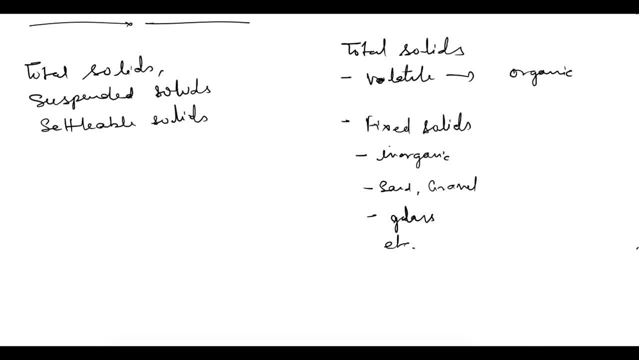 Whereas volatile solids will consist of organic matter, Which may be made up of fats and proteins. These all come in the volatile matter. So for the measurement, So for total solids, some sample is taken And then it is evaporated And whatever the residue is left. 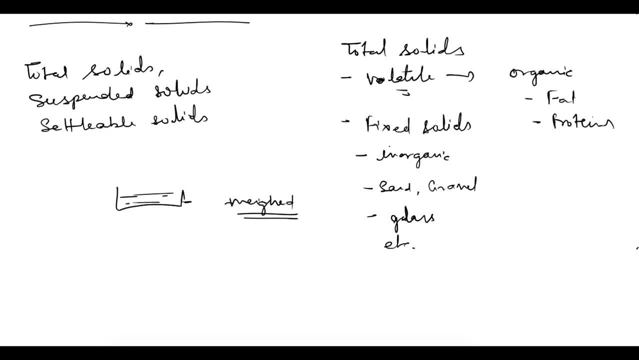 It is weighed. So that will give you the amount of total solids And if we divide it by the volume of sample, Then its concentration can be found out in the sample, In the waste water And for the volatile solid and fixed solids. 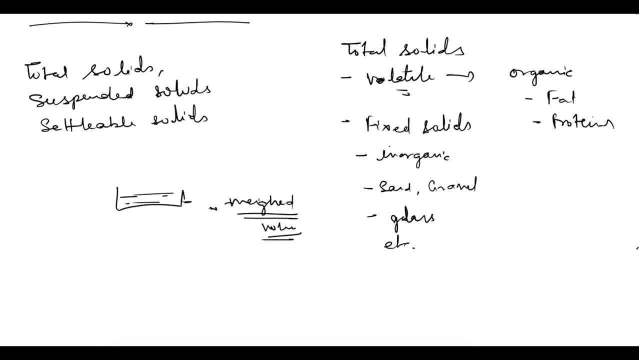 So this sample, whatever we have obtained after evaporation It is: initially it is heated to 103 to 105 degree Celsius For obtaining this total solids. After that the sample, whatever we have, I mean whatever is remaining after this evaporation, It is further heated up. 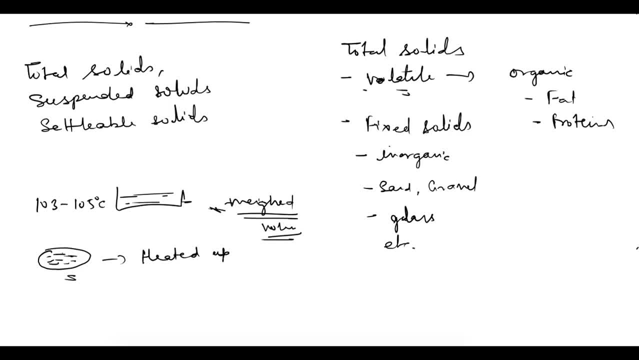 So in that process, this volatile matter is there. It will be burned Or it will be evaporated, we can say So. whatever will be remaining on this dish Or in the container, It will be your fixed solid, So we can take the total solid. 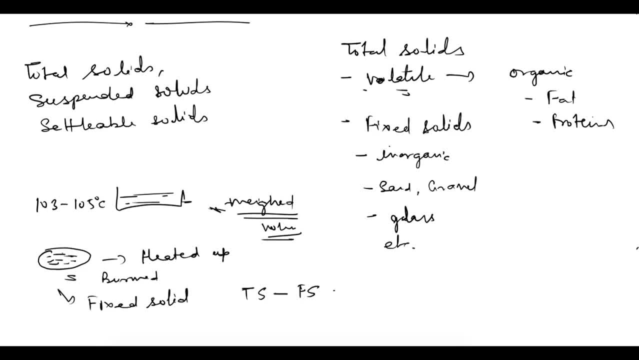 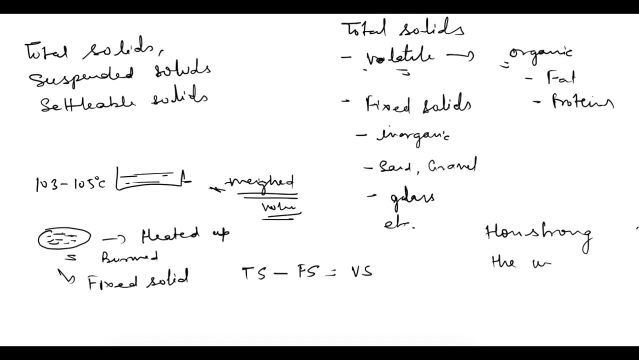 And minus the fixed solid, That will give you your volatile solids. So volatile solids Because these are made up of organic matter, So they give the idea that how strong the waste water is, Because this is the matter which has to be decomposed by organic matter. 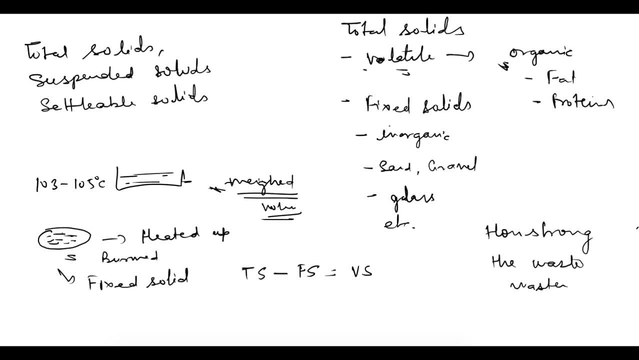 And by bacterial action and by oxidation process. So it will give you the idea of how strong the waste water sample is. If it is more, then it will be more strong waste water. That is for your total solids, And then we have suspended solids. 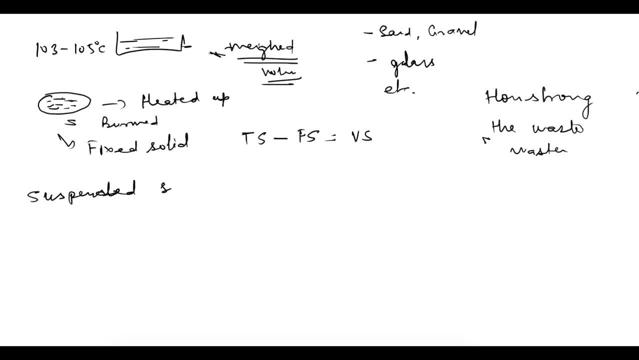 So suspended solids can be divided into two parts, That is, settlable solids And non-settlable solids. So to measure the total suspended solids, Some special lab filters are there And using them This size will be. Size of the filter would be. 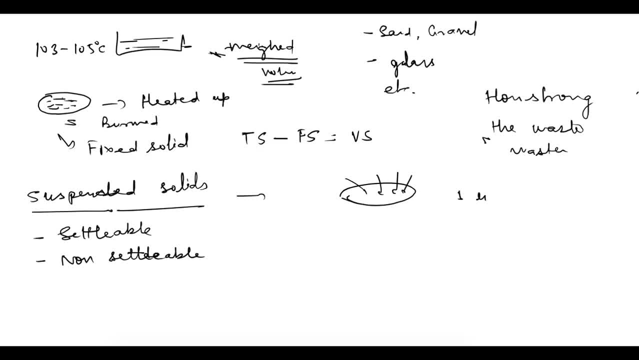 One, One milli, Sorry, one micrometer. So that is the size of this filter And using this, suspended solids can be filtered out And we can weigh this filter Or the residue which is left on it To find out total suspended solids. 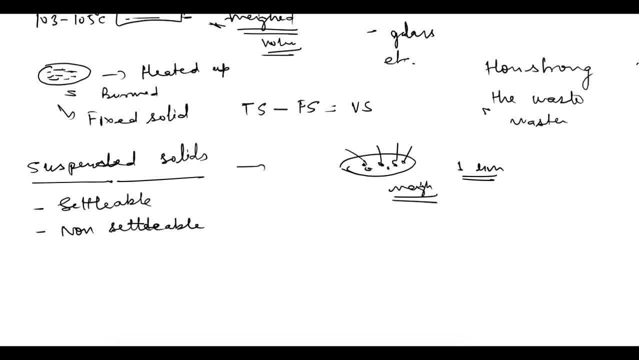 And for the settlable suspended solids Imhof cone is used. That is a conical equipment Or conical container, we can say So. the total volume that can come is one litre And these markings are there upto 50 ml. 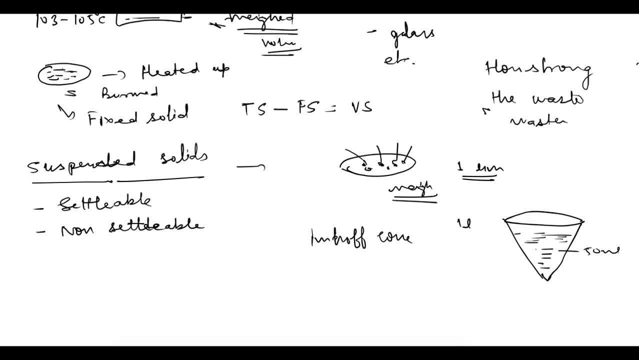 So water, This waste water sample is taken In this Imhof cone And it is allowed to settle for two hours And after this two hours, Whatever the solids that have settled Will give the approximate idea of this settlable solids. 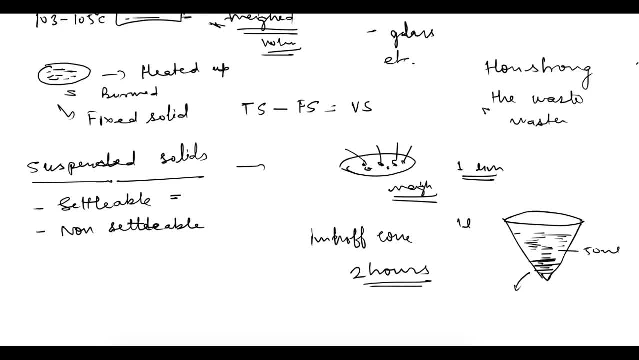 And for their proper measurement. This water, from upper layers It will be removed And whatever is remaining in the lower part It will be dried And it will be then weighed. So we can say it will be evaporated And then weighed. 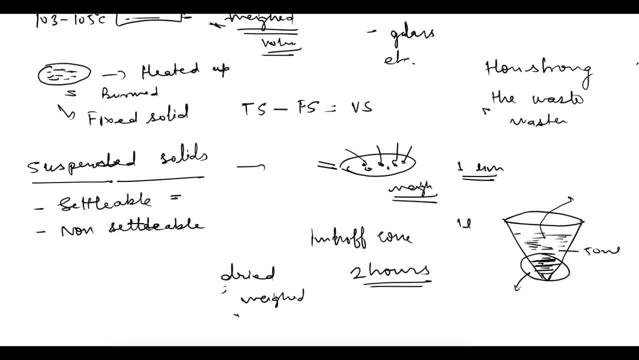 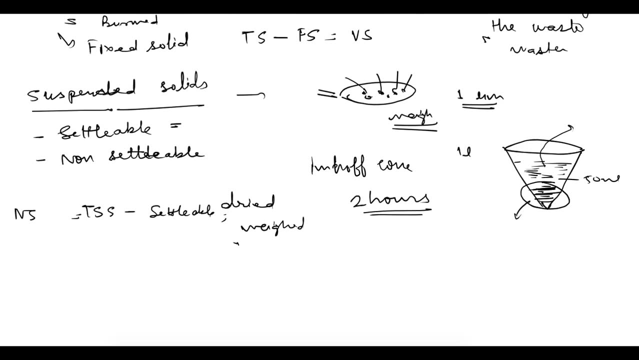 So that will give you the settlable solids, And from this filter we have obtained The total suspended solids. So total suspended solids Minus settlable suspended solids Will give you your non settlable suspended solids, Apart from suspended solids. 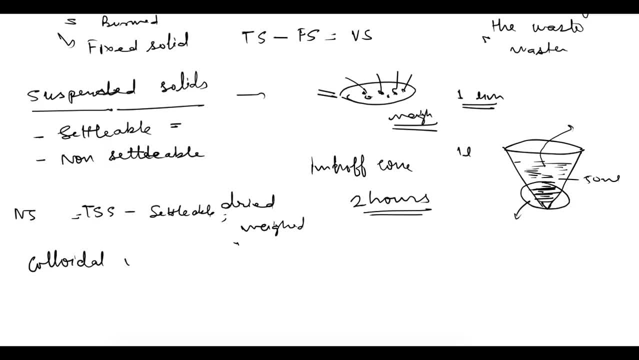 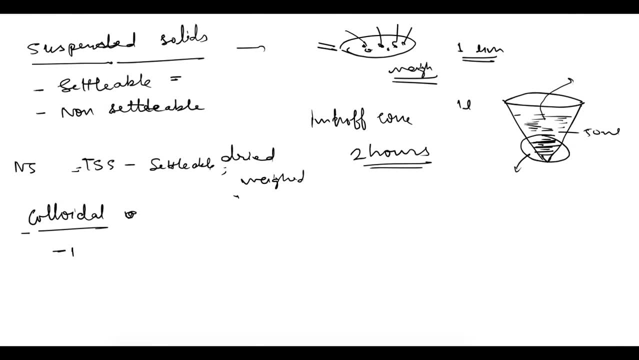 Some colloidal particles will be present in the water, So these cannot be filtered out Using some filter, Because this particle size is very small: It is between 1 millimicron to 1 micron. So these are. These can be filtered out. 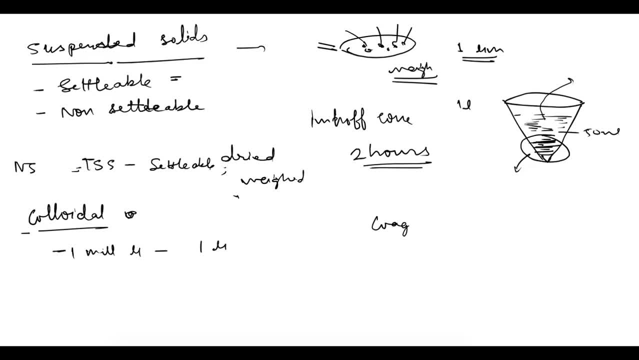 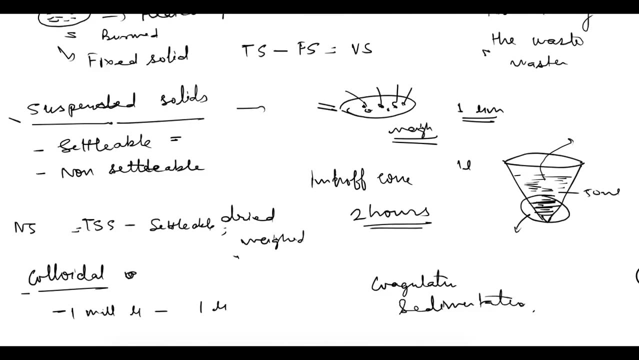 And for their removal, We can simply, As we did earlier, We can do the coagulation and sedimentation And for the measurement, Obviously we can, If we can find out the total solid And suspended solid. So whatever is remaining, 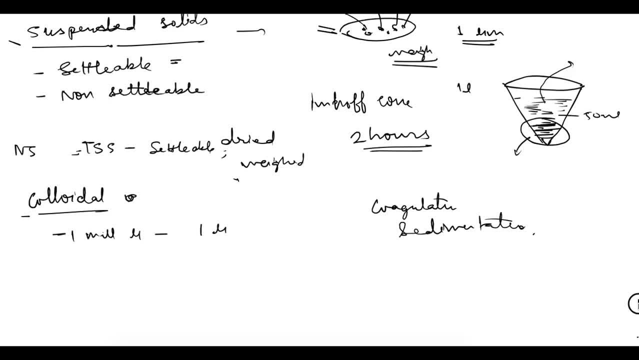 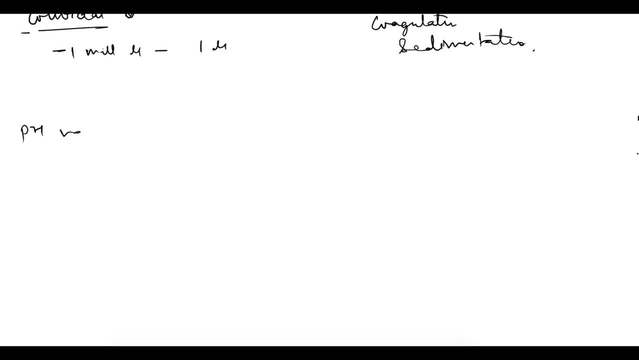 That will be your colloidal solid After this. Next parameter we have is pH. So pH of wastewater, If it is a fresh sewage, Then pH is on alkaline side. That is between 7.2. Or we can say 7.2 to 7.5.. 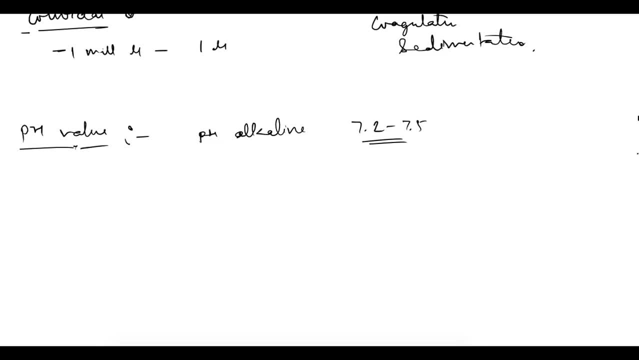 This will be the range for the pH Initially, If it is a fresh sewage And due to the- I mean after some time- Due to the production of Acid, And that acid will be produced Due to this bacterial action. So these bacteria produce these acids. 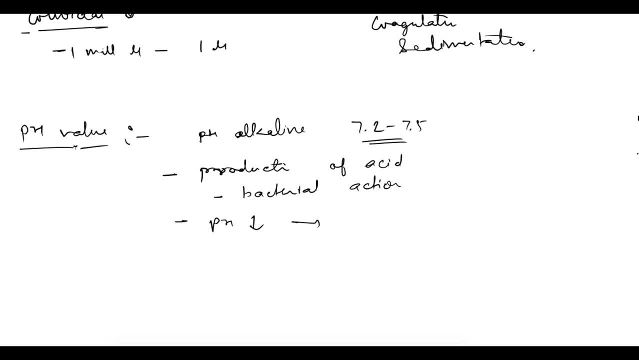 And the pH starts to go down. So when the decomposition is taking place, Then this wastewater pH is on the acidic side, And after the decomposition- Or we can say The oxidation is complete- Then again the pH comes on the alkaline side. 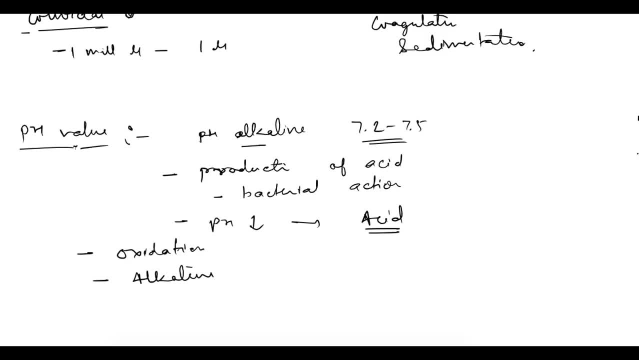 So using this We can find out whether the pH is. I mean, if we can see the color And pH, Then we can tell If it is a recent Pollution, I mean recently Used wastewater, Or it is a old wastewater. 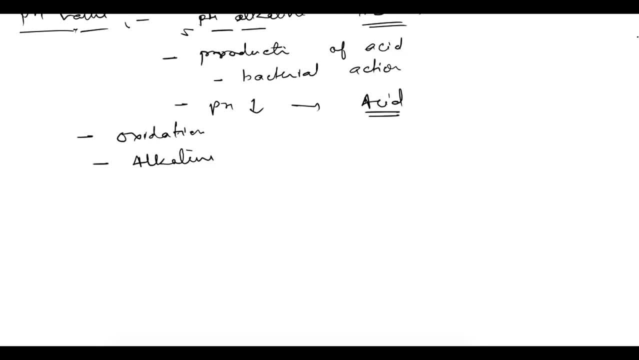 After pH Next. Apart from that, One more thing that is there in pH is: If pH is very low Or very high, It will tell you that It is. I mean, this wastewater is coming from Some industry. After pH next. 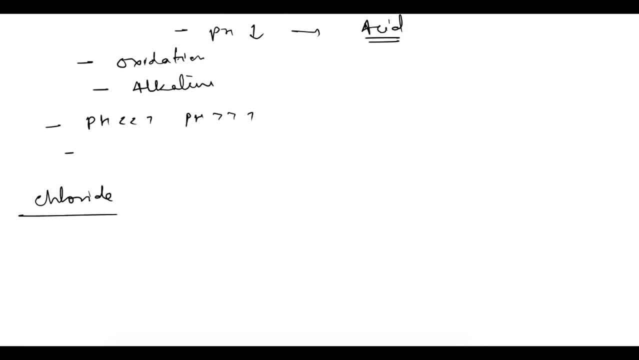 We have chlorides, So chlorides in wastewater come Can come in from domestic sources And from industrial sources also From domestic sources Because salts and all Is there We use in kitchen. So That can be the one of the reasons. 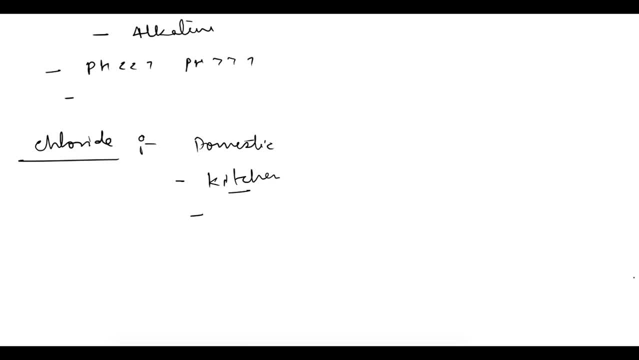 Of This chlorides. Apart from that, Human excreta And Urine Both have chloride in it. So If it is a domestic waste, Then 120 milligram per liter Is the Normal consumption, Normal concentration. 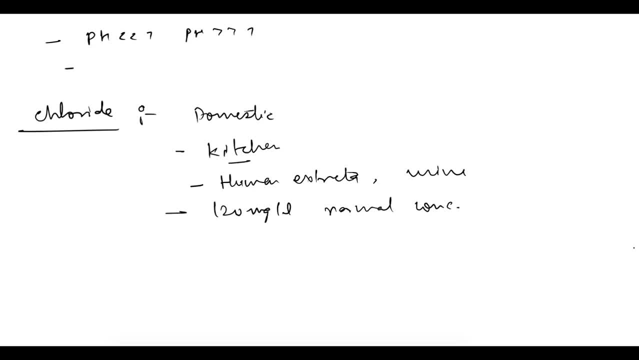 That can be found out In wastewater. If it is a domestic waste- And for the industries It is- It comes due to ice cream plants. Apart from that, If some Industries Are, factories, are there Where salts Are used highly? 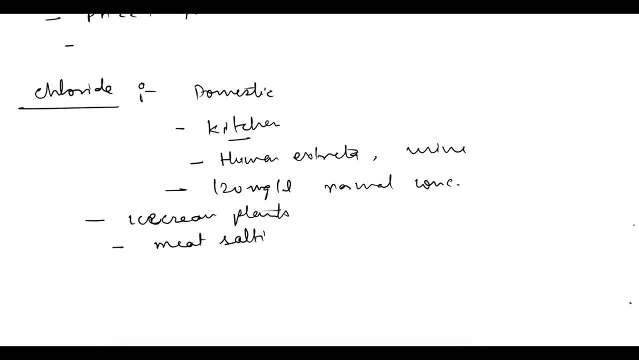 So for meat, salting It It, This chloride will be more From that industry And apart from that, Some, If some infiltration is happening. This infiltration Can be there Due to sea water Or If some groundwater. 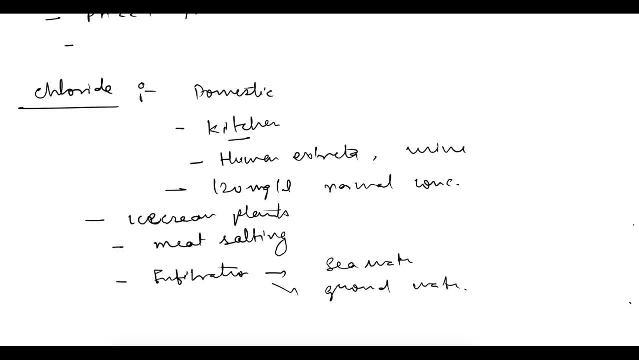 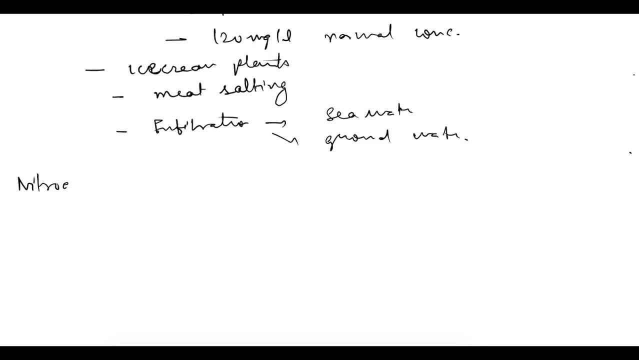 Is there Which is high In chloride, Then Due to these reasons Also, Chloride can come in Wastewater. Next We have is nitrogen Contain For the measurement Of chloride, Similar to the What? 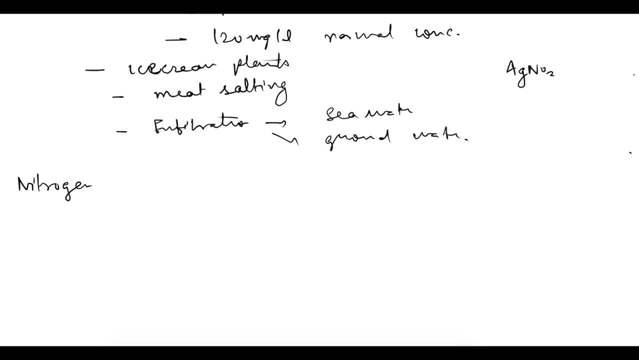 I mean, We have already seen In water supply We use The silver nitrate solution And We do the titration. That way We can measure the Chloride. Next Is nitrogen Contain. So this also. 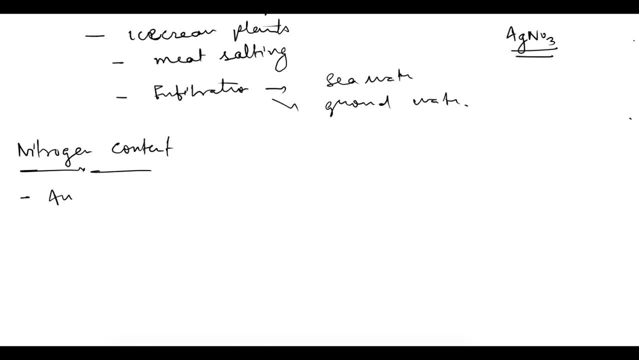 We have seen in The water treatment. From there You can see In detail. So nitrogen Is present In various forms. That is, Ammonia Can be there, Organic nitrogen Can be there And then Nitrites. 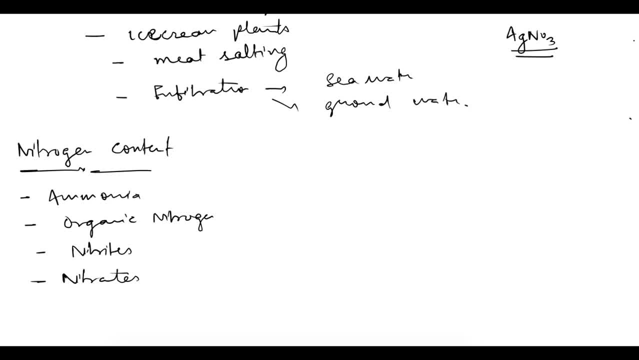 Can be there And Nitrates Can be there. So they will tell you The different stages Of decomposition. If ammonia Is present, That means It is a Fresh wastewater. None of the Organic, I mean. 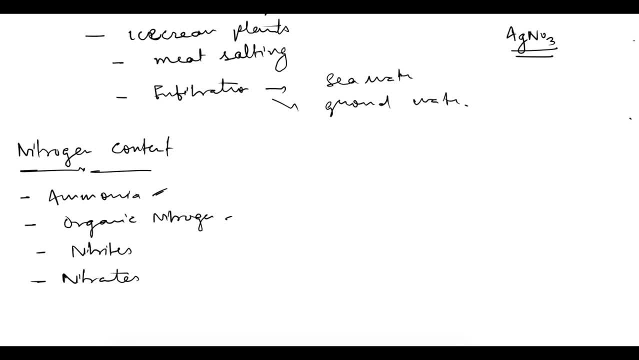 The organic matter Has just started Decomposition, Decomposing And For Organic nitrogen. It will Give you The idea Of How much Undecomposed Organic matter Is present. Nitrite Will tell. 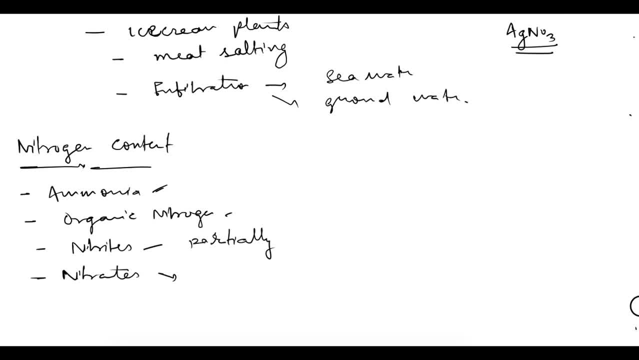 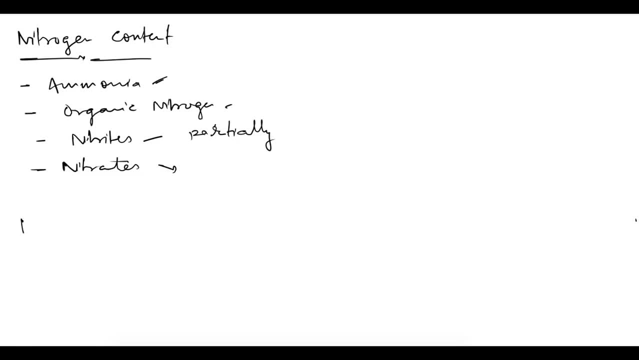 The amount Of Partially- I mean Partially- Decomposed Organic matter Is Completely Decomposed. That Is Your Nitrogen Content. Then We Have These Fats Grease.